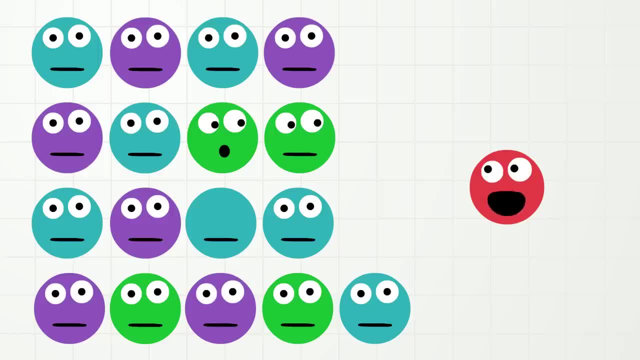 Hey, who is talking? Francis and August, please be quiet. Okay, as I was saying, I want to observe my brothers and sisters and collect data Data about what color they are. Do you want to help me? Okay, great, We can use a chart. 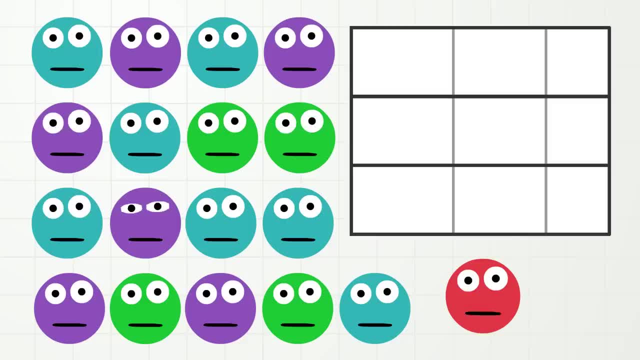 and write down the numbers beside the words of the color up here. First up is purple. So how many brothers and sisters are purple? Let's count One, two, three, four, five, six, Six. Hey, do you know what these are? 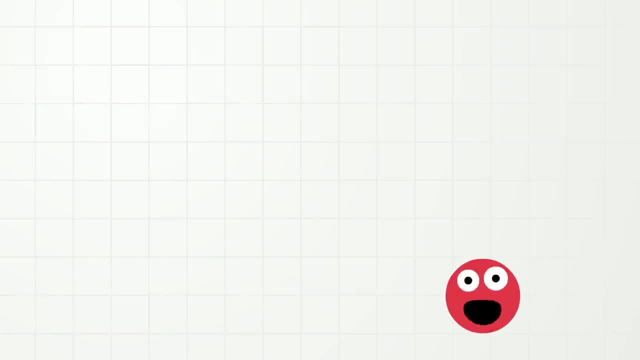 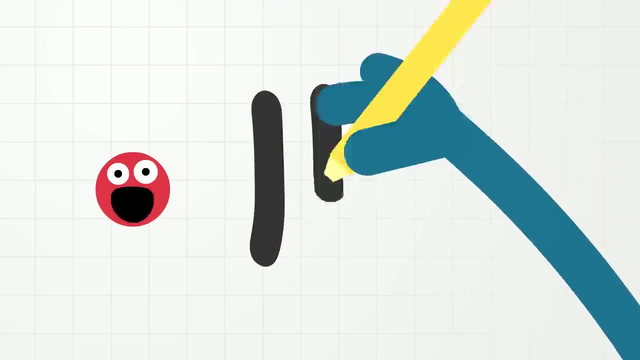 These are tally marks, Tally marks. Tally marks are like a way of counting using special lines. When we count with tally marks, we make one up and down line for each number, up to four, like this. And then, when we get, 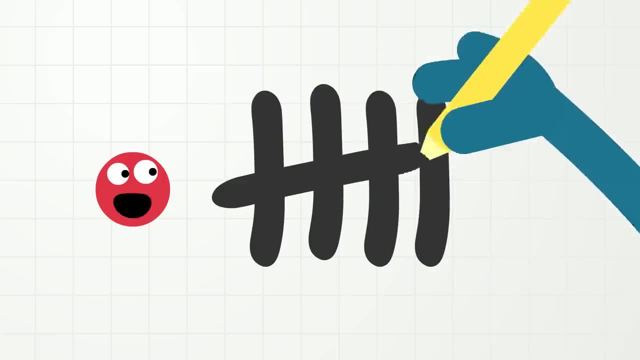 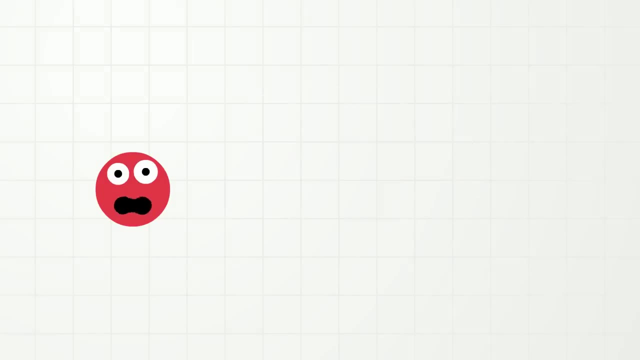 to five. we make a side to side line through like this, And now we know we have a group of five, But after five, Well then we start all over again, All over again and make a new group, So when we count up to six. this is how we do it with. 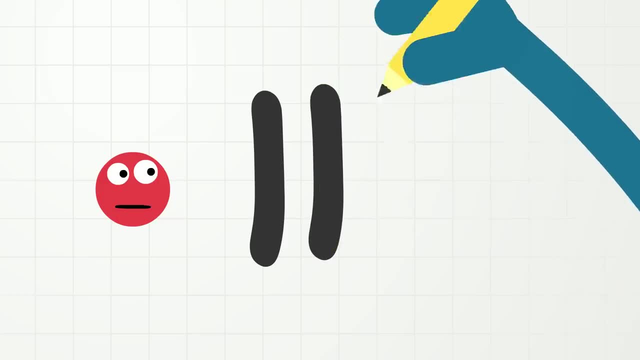 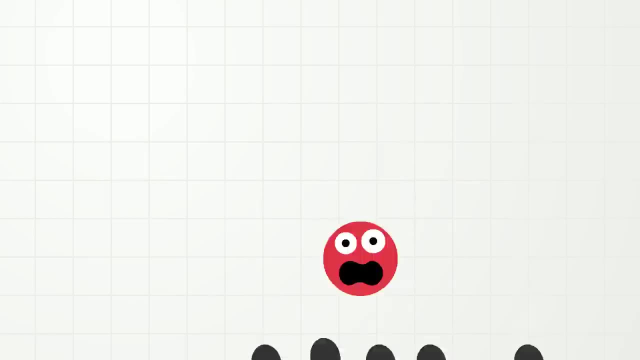 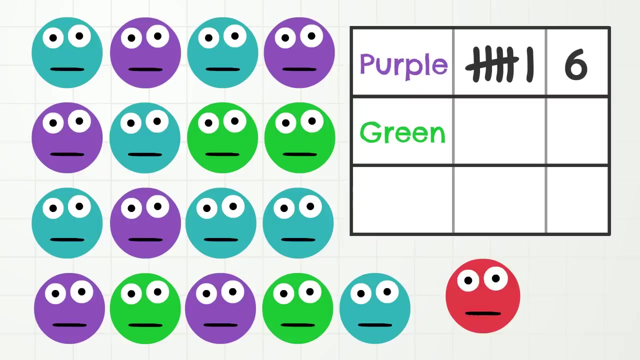 tally marks One, two, three, four, five and six. Okay, moving on, The next color is green. How many brothers and sisters are green? Let's count One, two, three, four, five, six, seven. And finally, how many brothers and sisters are blue, Let's count One, two. 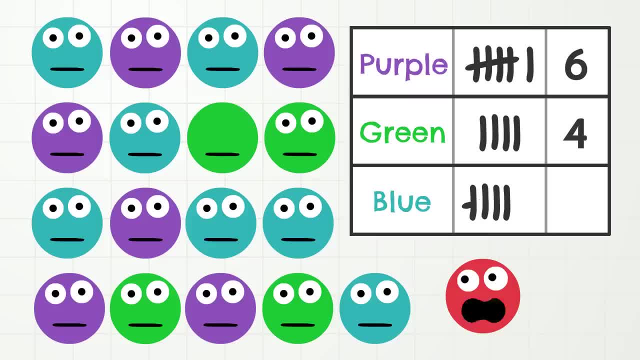 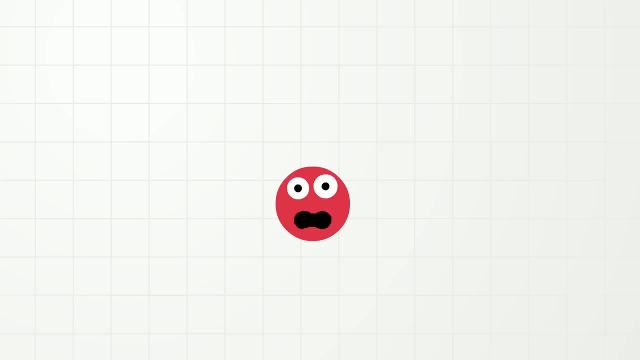 three, four, five, six, seven, Seven. Good job everybody. We have now collected all the data about the color of my brothers and sisters. Yay, Okay, you've done such a good job. It is now time to take a stretching break. Ugh, Yeah, Okay, that's enough. So we just saw. 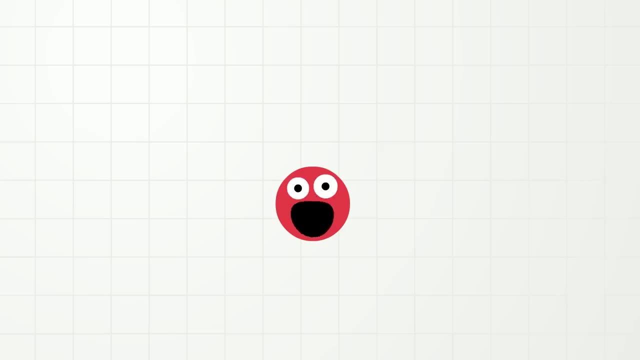 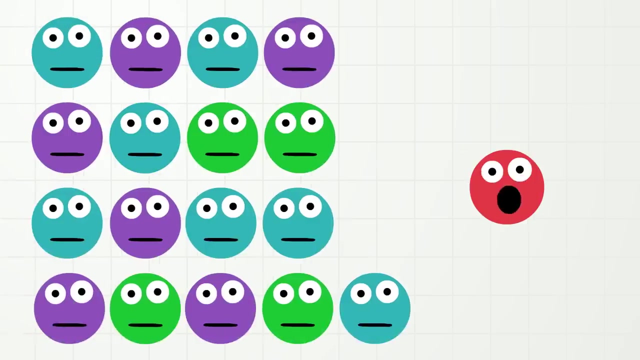 that we can collect data and understand things by observing with our eyes, But did you know that we can also collect data and understand things by asking questions with our voice? Oh, yes, we can. Okay, let's ask my brothers and sisters some questions and collect their. 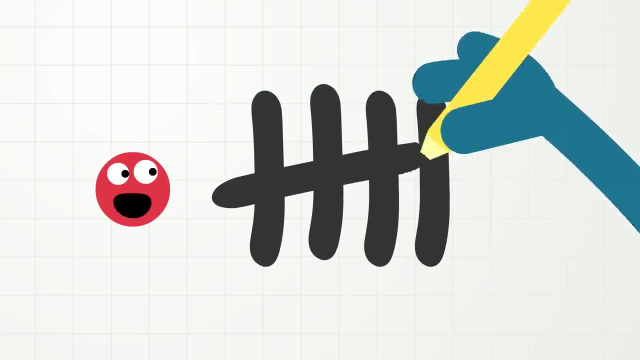 to five. we make a side to side line through like this, And now we know we have a group of five. But after five, Well then we start all over again. We start all over again and make a new group. So when we count up to six, this is how we 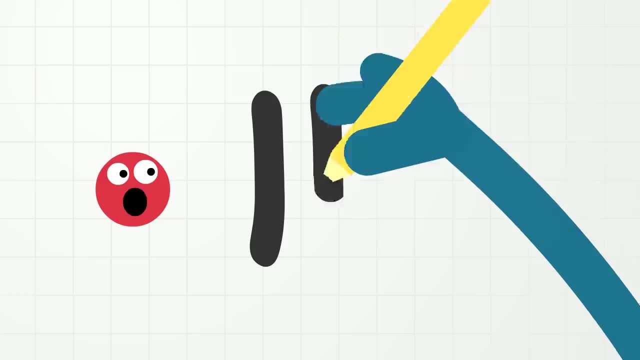 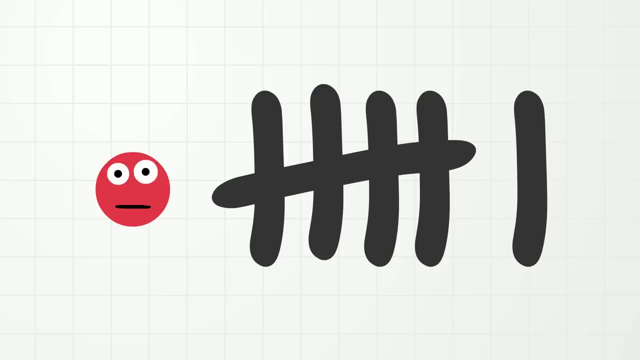 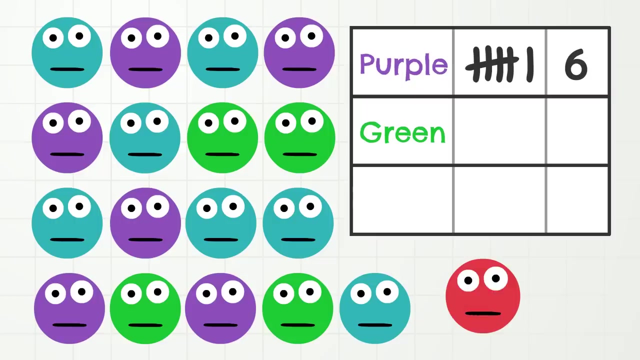 do it with tally marks One, two, three, four, five and six. Okay, moving on, The next color is green. How many brothers and sisters are green? Let's count One, two, three, four, four. And finally, how many brothers and sisters are blue, Let's count One, two, three. 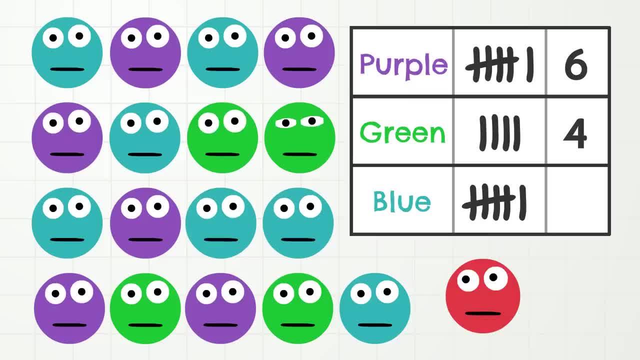 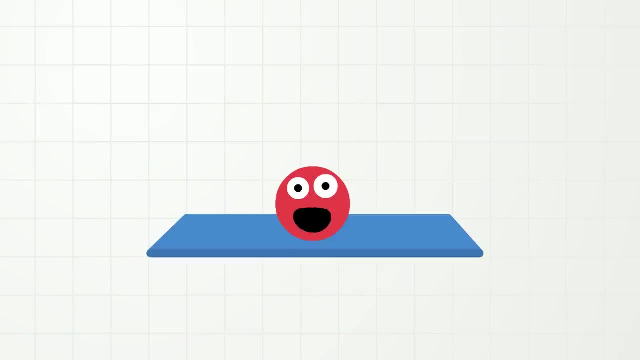 four, five, six, seven, Seven. Good job everybody. We have now collected all the data about the color of my brothers and sisters. Yay, Okay, you have done such a good job it. It is now time to take a stretching break. 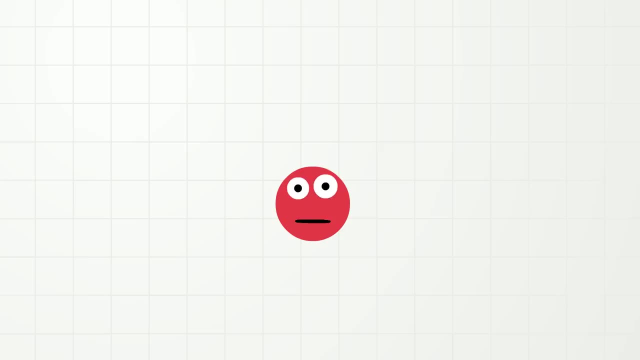 Ugh, Yeah, Okay, that's enough. So we just saw that we can collect data and understand things by observing with our eyes, But did you know that we can also collect data and understand things by asking questions with our voice? Oh, yes, we can. 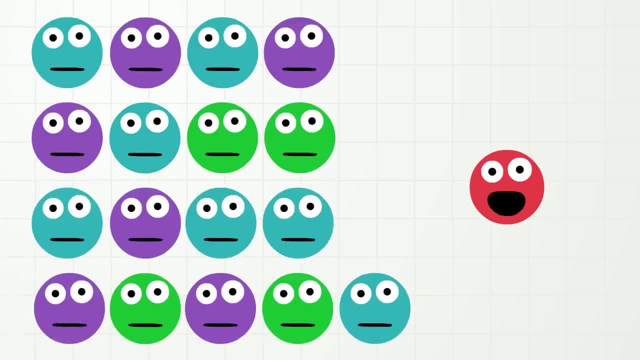 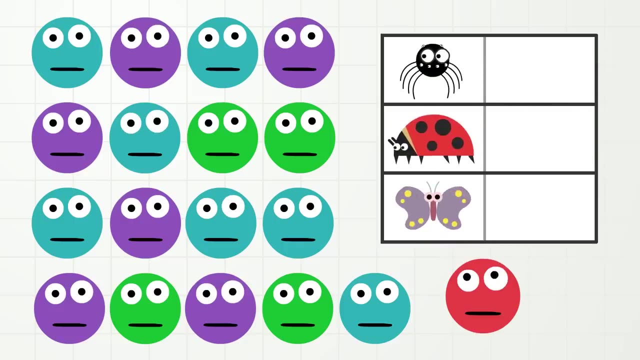 Okay, let's ask my brothers and sisters some questions and collect their answers with tally of bugs. Okay, what should we ask them about? Hmm, Oh, I know Bugs. I said bugs. Okay, there are three different kinds of bugs here. 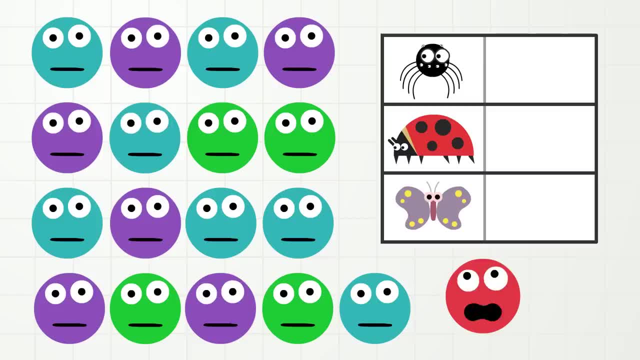 Spider, ladybug and butterfly. I want to know which bug they like the best. So we just saw that…. Hey, who's talking? Ugh, Jesus and August, You need to separate, Please move. Okay, that's better. 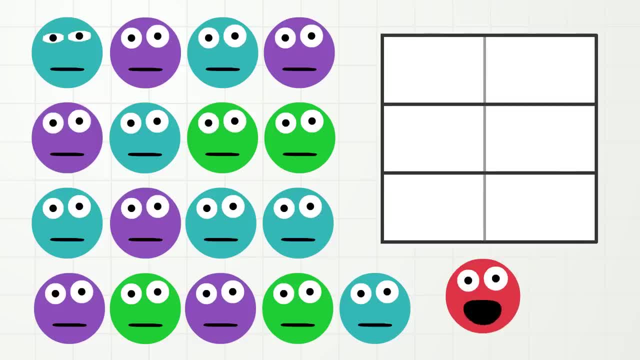 answers with tally marks. Okay, what should we ask them about? Hmm, Oh, I know Bugs. I said bugs. Okay, there are three different kinds of bugs here: Spider, ladybug and butterfly. I want to know which. 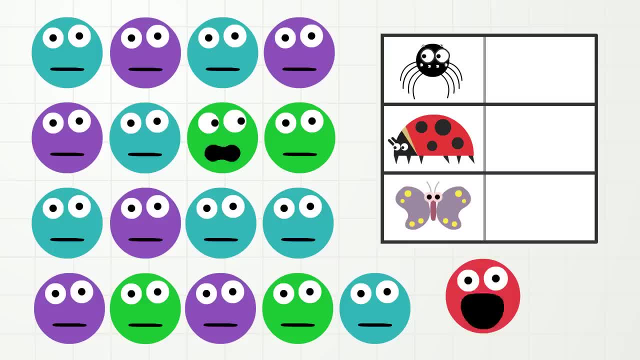 bug they like the best. So we just saw that. Hey, who's talking? Ugh, Francis and August, You need to separate, Please move. Okay, that's better Now. brothers and sisters, I want you to raise your hand when I say the name of the bug that you like the best And remember. 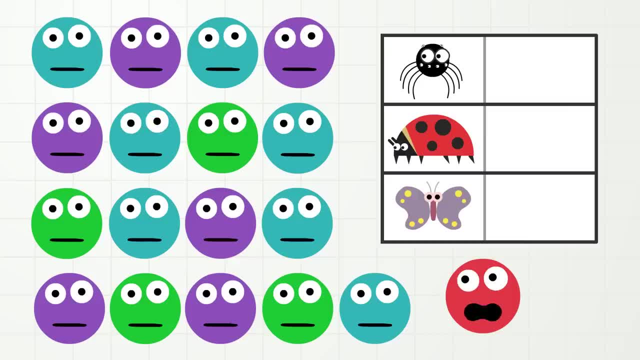 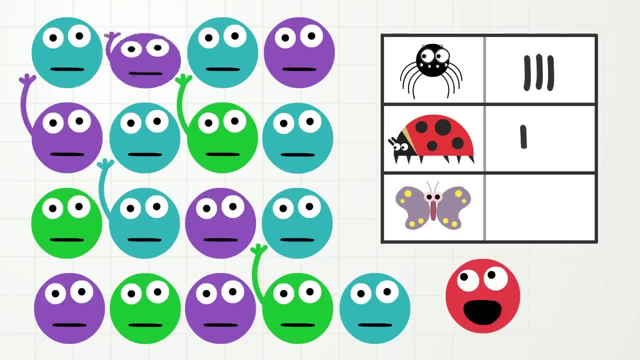 a ladybug's the best, Let's count. One, two, three, four, five, So five, brothers and sisters. like a ladybug's the best, Now raise your hand if you like. a butterfly's the best, Let's count. 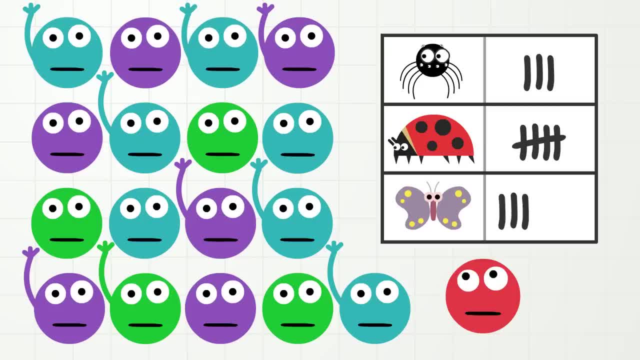 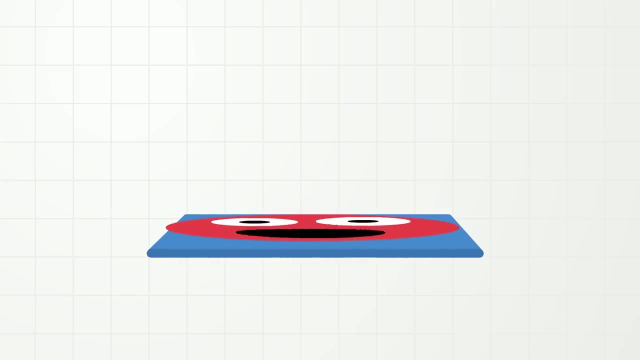 One, two, three, four, five, six, seven, eight, nine. So nine brothers and sisters. like a butterfly, the best, Wow, great, collecting data everyone. Now let's take a break and do some stretching. Oh yeah, feels good. Okay, that's enough. Now let us show this data in a different 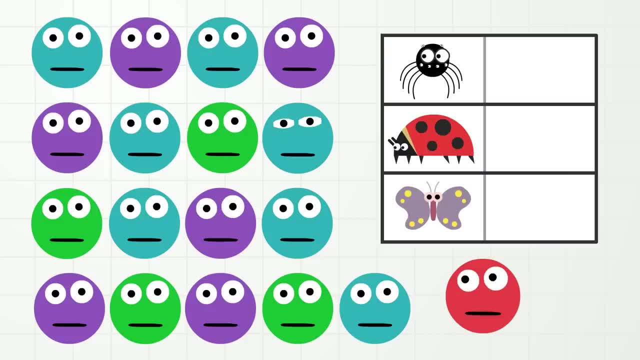 Now, brothers and sisters, I want you to raise your hand when I say the name of the bug that you like the best. And remember you can only choose one bug and raise your hand one time. Okay, please raise your hand if you like spiders the best. 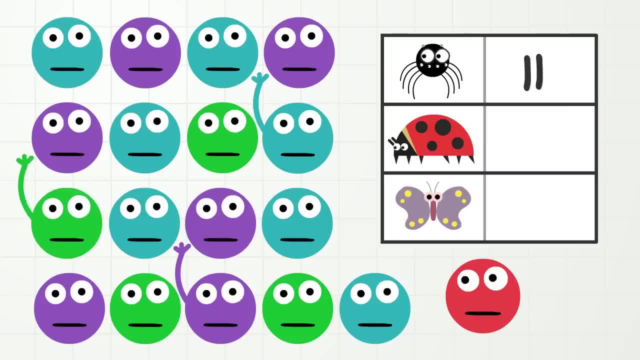 Let's count One, Two, Three, So three brothers and sisters like spiders the best. Now raise your hand. if you like ladybugs the best, Let's count One, Two, Three, Four, Five, So five brothers and sisters like ladybugs the best. 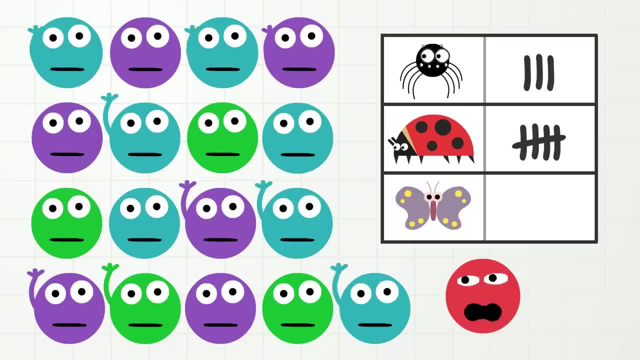 Now raise your hand. if you like butterflies the best, Let's count One, Two, Three, Four, Five, Six, Seven, Eight, Nine. So nine brothers and sisters like a butterfly the best. Wow, Great, collecting data everyone. 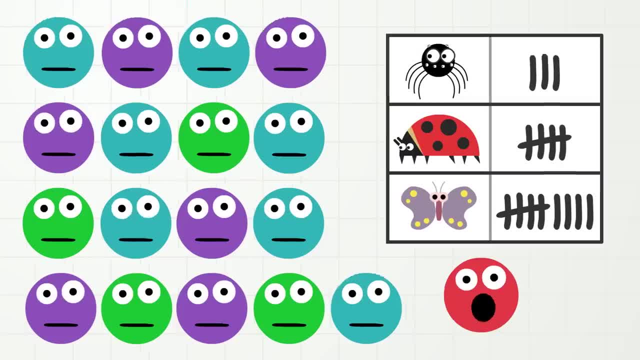 Now let's take a break and do some stretching. Ugh Yeah, Feels good. Okay, that's enough. Now let us show this data in a different way. Let's take a break and do some stretching. Oh Yeah. 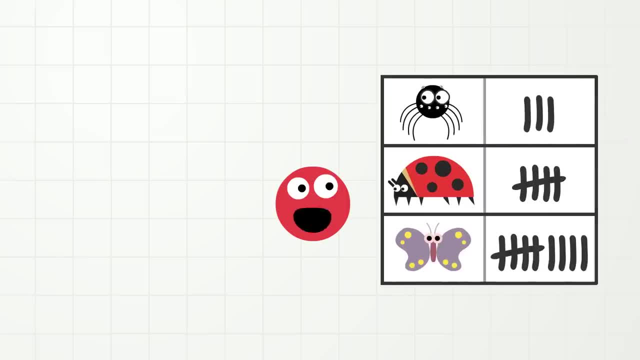 Feels good. Okay, that's enough. Now let us show this data in a different way. Okay, that's enough. Now let us show this data in a different way. Instead of using tally marks, we will take the numbers and put them into something we 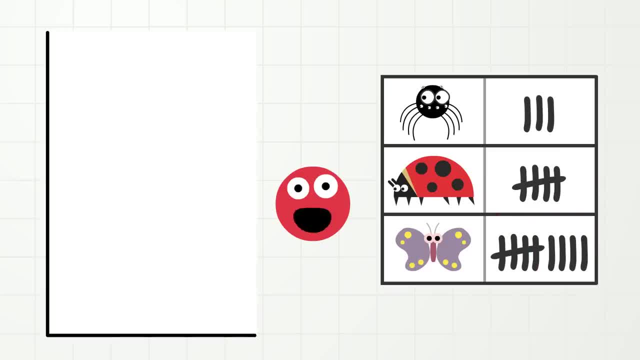 call a pictograph Pictograph. A pictograph is a way to show data with pictures. Okay, so remember how many brothers and sisters liked spider best- That's right, three, One, Two, Three. And how many liked the ladybug the best. 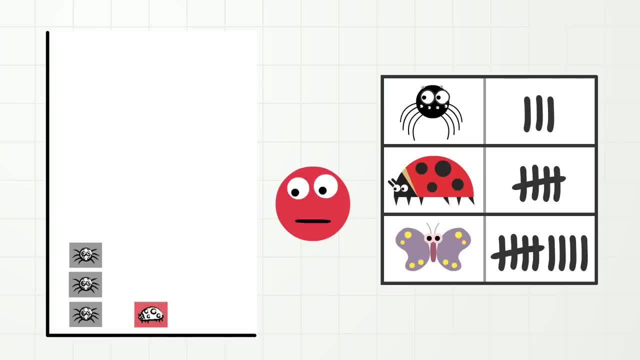 That's right: five, One, Two, Three, Four, Five. And how many liked the butterfly the best? That's right: nine. One, Two, Three, Four, Five, Six, Seven, Eight And nine. And now our pictograph is complete.